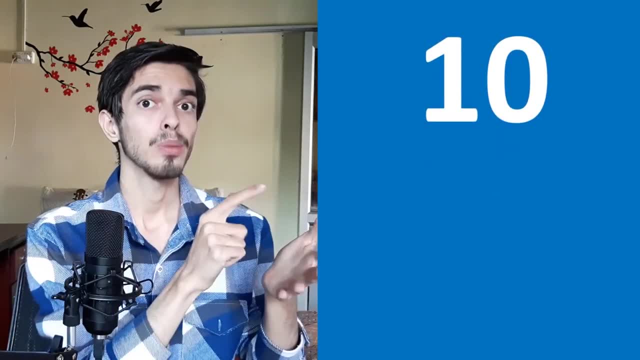 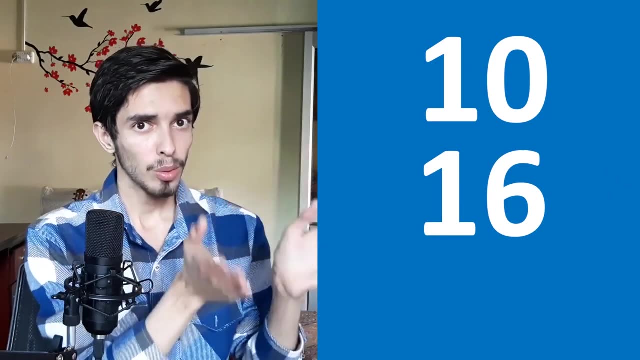 down, So 10.. Now we have subtracted 3 from 13.. So add 3 in 13., So 16.. Now we have 10 and 16. Now multiply these two, So 16 times 10 is 160, which is very simple. Now in this 160,. 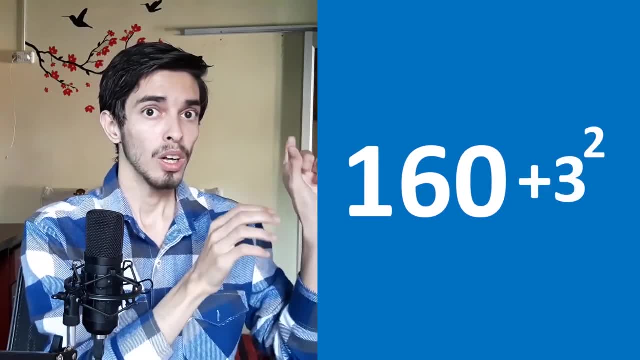 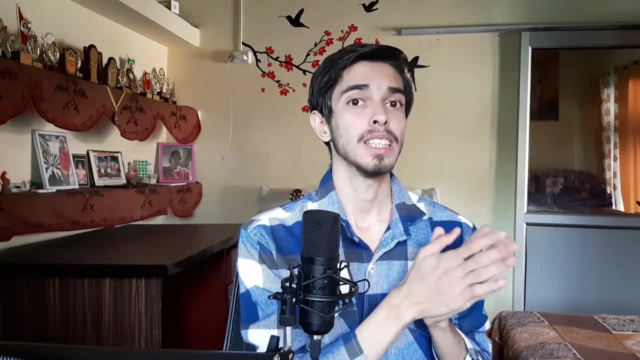 you just need to add the square of 3, which we have subtracted. So 160 plus 9 is 169,, which is the square of 13. And this is how you can square any two-digit number. Now try 12.. 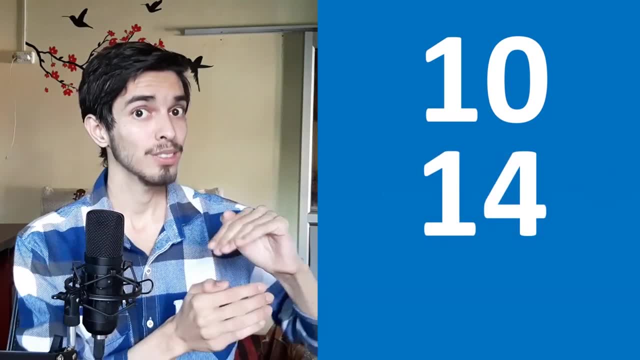 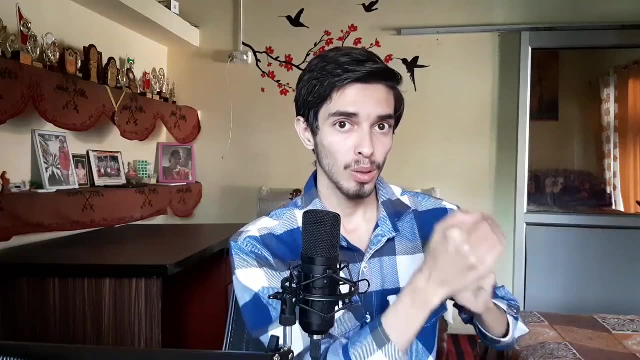 So round down 10, multiply by 14.. 140 and 2 square is 4.. So 144 is our answer. So this is how you can square any two-digit number. Now let's try 19.. This is a little bit difficult. 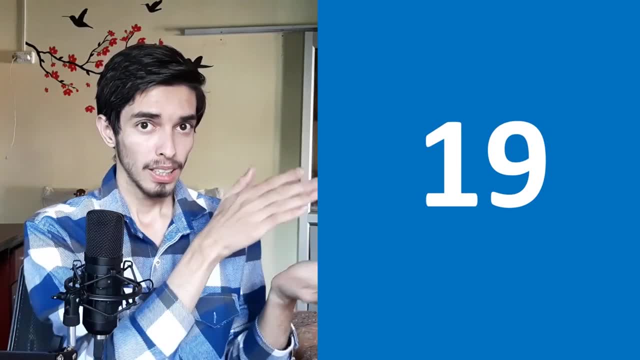 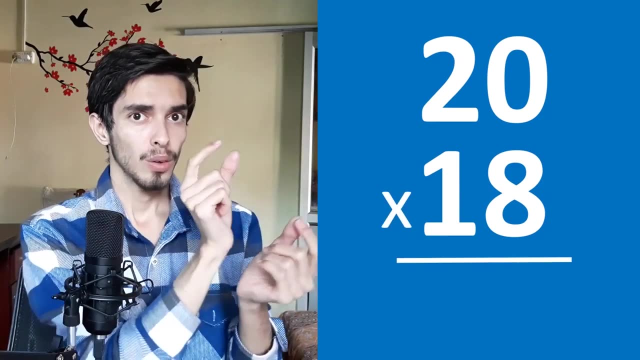 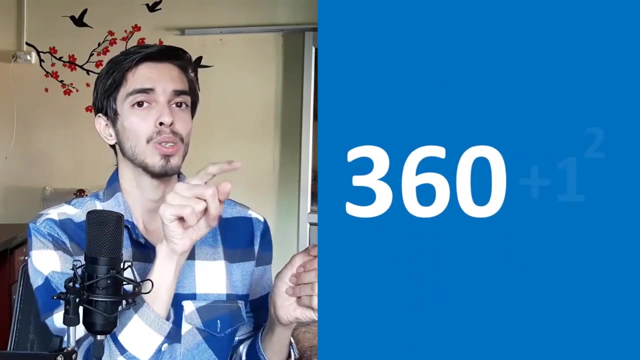 because there will be a 20 here, Okay, but don't worry. So 19 round up 20.. 1 round down 18.. So 18 times 20.. Now, 18 times 2 is 36.. So 360.. Now in here we just need to add 1 square. 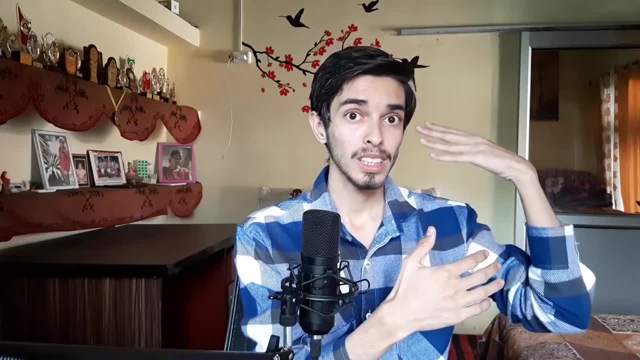 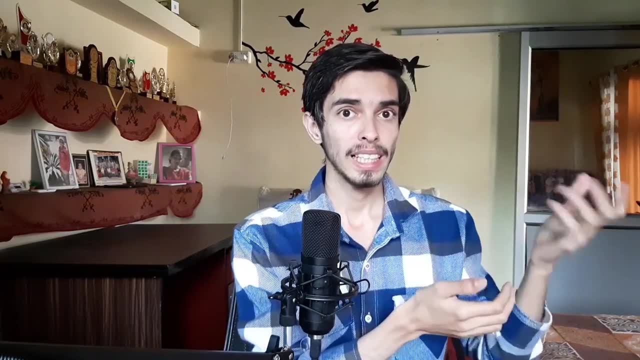 which is 1.. So 361 is our answer. So see, you have just done 19 square. That is 19 times 19 in your head right now, in here. Now you can take any number from 11 to 19 in here You can. 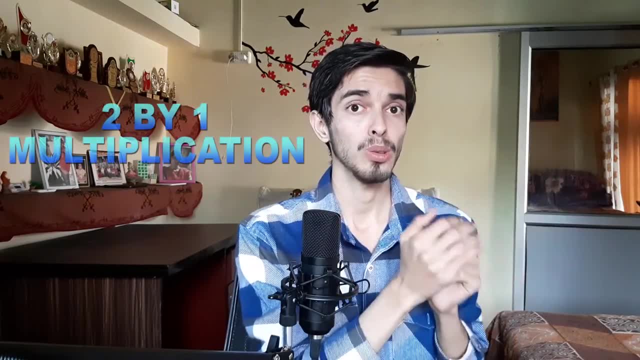 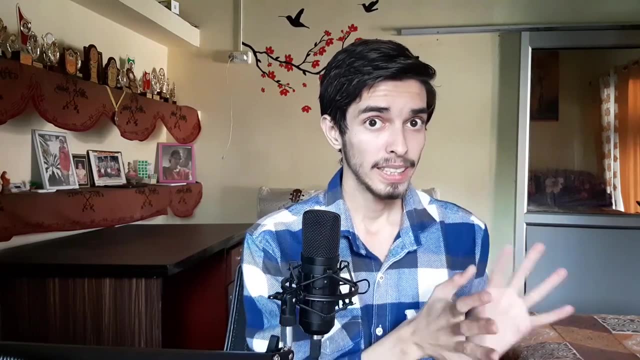 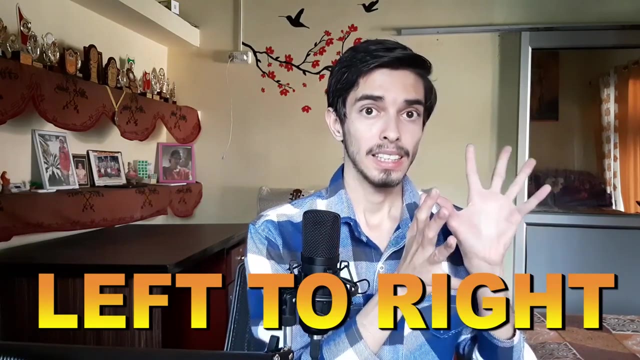 go further, but it would be a little bit difficult. For that, you need to learn 2 by 1 multiplication. So let's learn 2 by 1 multiplication, which is very simple. Same method here as we did. in addition and subtraction, Always go from left to right, And if you have watched those videos, 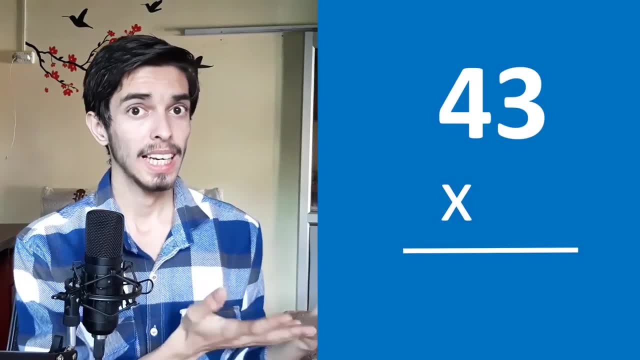 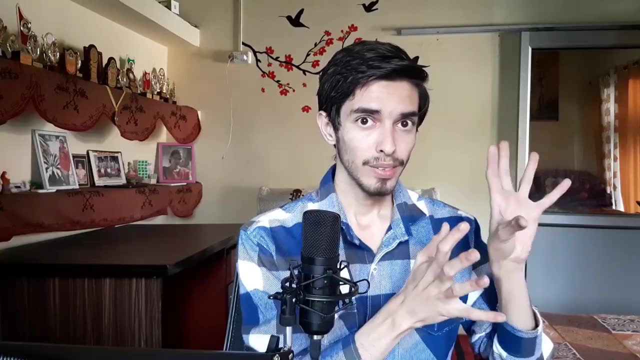 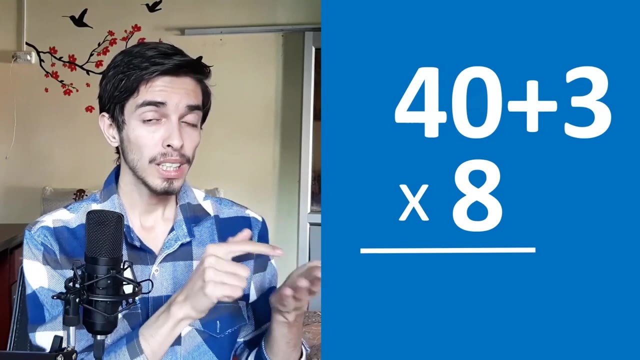 you will know what is its benefits. So let's multiply 43 and 8.. Now, instead of multiplying 3 with 8, then taking carry, then 4 with 8, and then adding, we will go the easier way, the left to right method. So 40 times 8 first. So 40 times 8 is: 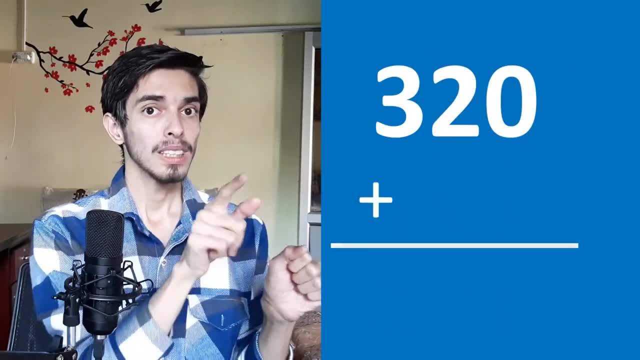 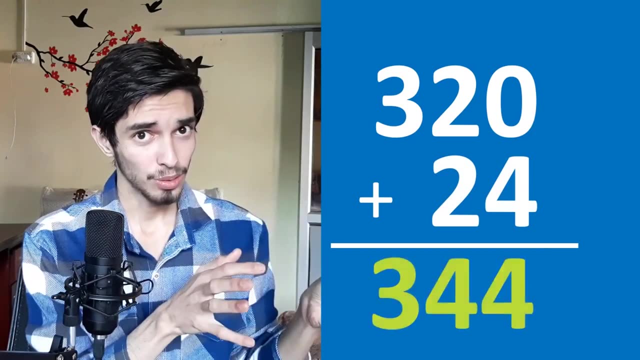 8 times 32.. So 320.. Now 3 times 8,, which is 24.. So 320 plus 24 is 344.. So this is the basic 2 by 1 multiplication. So in this problem we converted 43.. 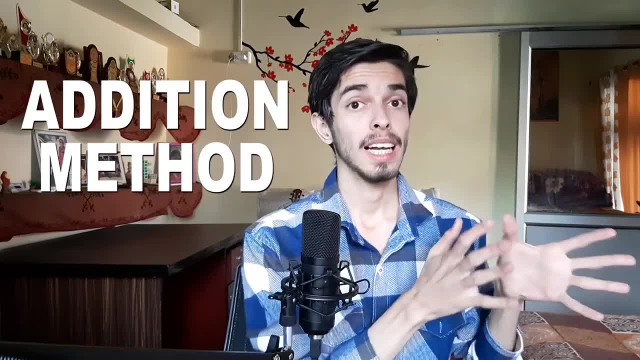 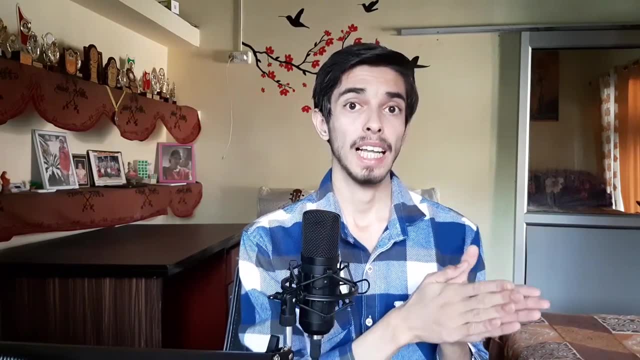 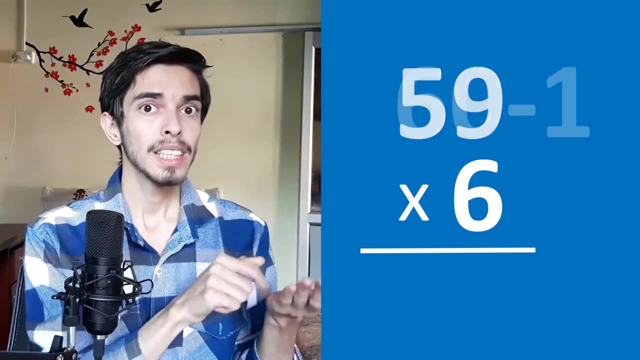 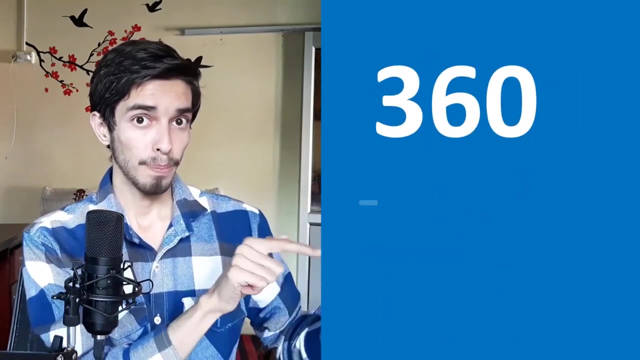 This is known as the addition method for multiplication. The other method is the subtraction method. It is used for problems like this: 59 times 6.. Now, instead of going like 50 plus 9,, we will do this 60 minus 1 times 6.. So 60 times 6 is what 6 is 36.. So 360 minus 6.. So 60 times 6 is what? 6 is 36.. So 60 times 6 is 36.. So 60 times 6 is 36.. So 60 times 6 is 36.. Now, after learning this 2 by 1 multiplication, you have also learned something else. 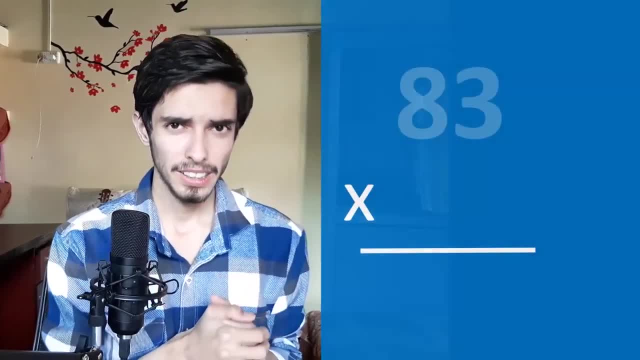 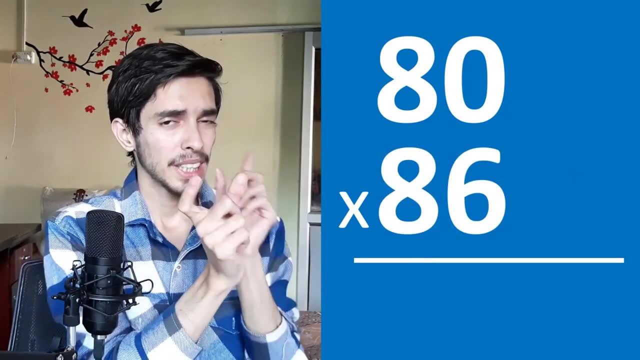 the square of any two-digit number. So for example, 83 square. Now round down 80 times 86.. Now this 80 times 86 seems 2 by 2 multiplication, but it is just 86 multiplied by 8 with a 0.. 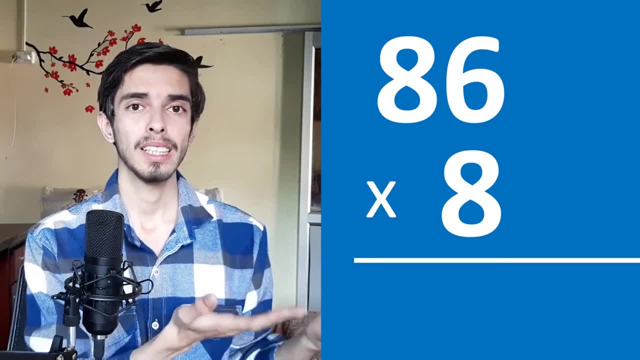 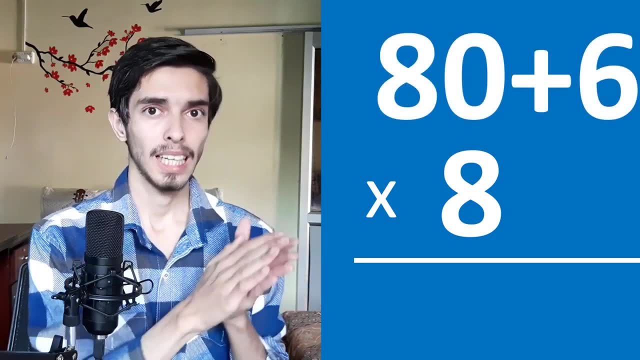 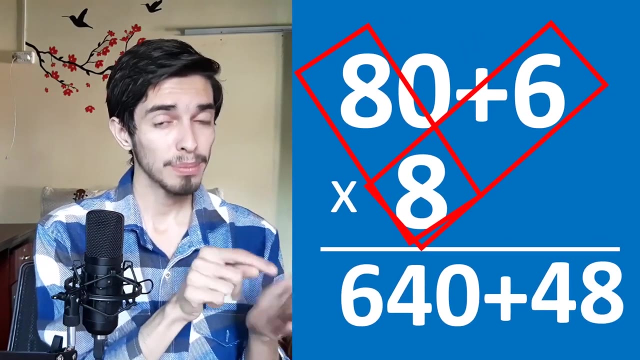 You can do this problem either by addition method or subtraction method. It's your choice. So I will go with addition method. So 86 times 8.. So 80 plus 6 times 8.. So 8 8s are 64.. 6 40 plus 8 6s are 48.. So 6, 40 plus 48.. So 6 40 plus 48 is 6, 88.. And we have a 0. 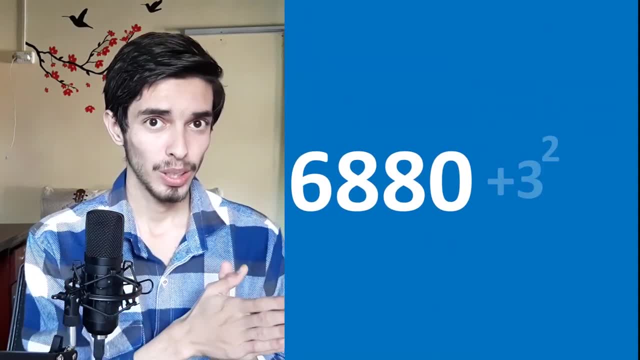 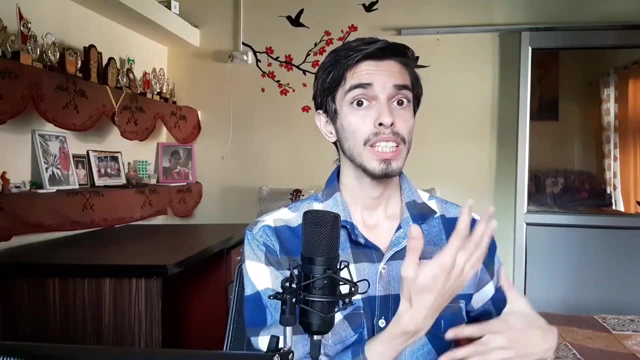 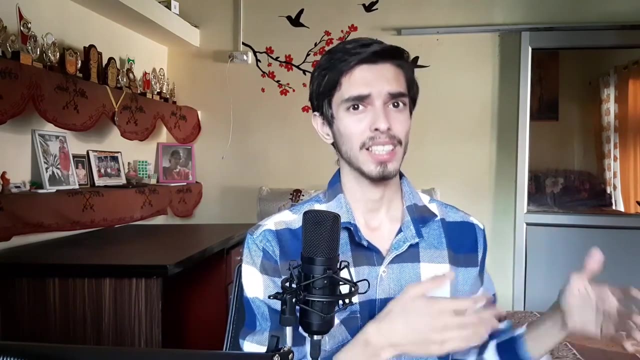 also. So 6, 8, 8, 0.. So, adding just 3 square in here, which is 6, 8, 8, 9,, which is the square of 83.. So see, you are able to do this. You have just done the square of 83 in your head, which is insane. 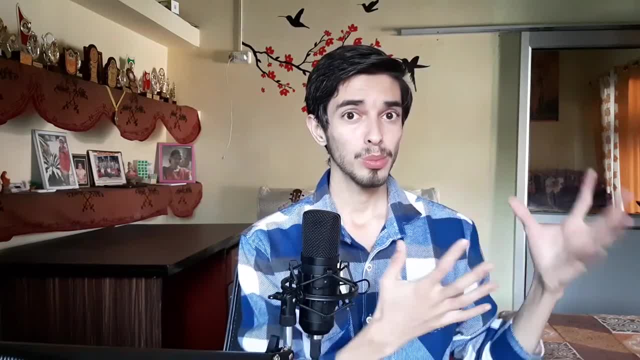 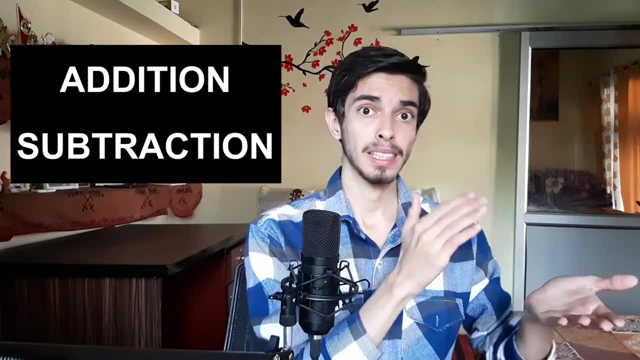 Now let's go with 2 by 2 multiplication. Now, 2 by 2 multiplication is really interesting, because there is the addition method of multiplication, There is the subtraction method of multiplication And there is also another method known as factoring method. Also, 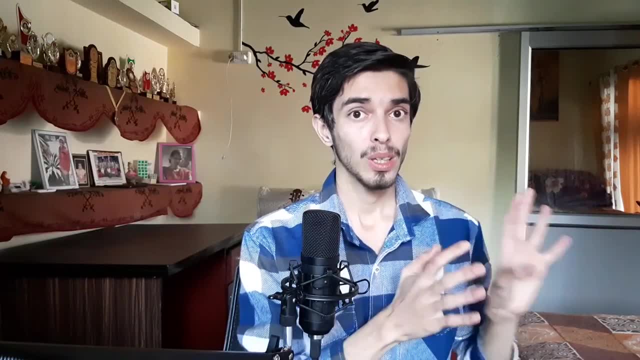 you can also mix these methods together to get creative, And also remember that the more creative you are, the more creative you are. So you can also mix these methods together to get creative. So you can also mix these methods together to get creative, And also remember that the more creative 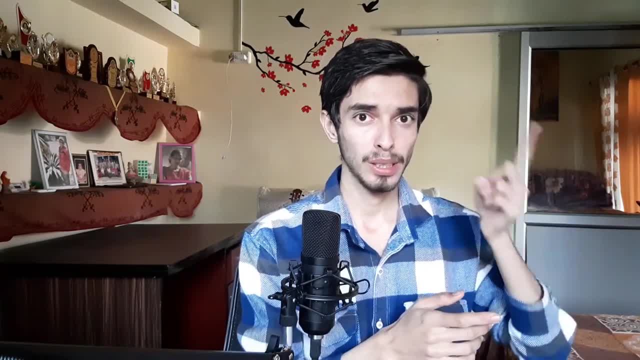 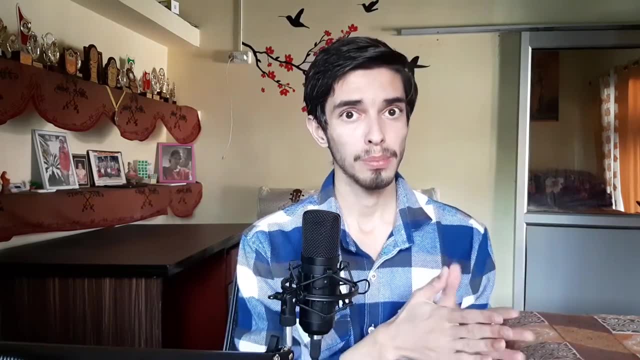 you are, the faster you will be. So let's take one problem and do it with all three: addition, subtraction and factoring methods. After that, the more you will practice, the better you will become. And also, in 2 by 2 multiplication, the factoring method is the best. You will see that. 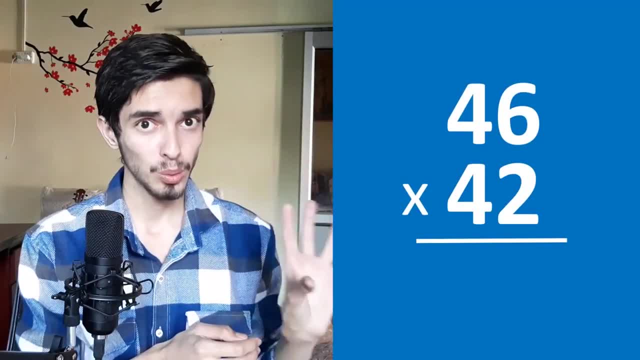 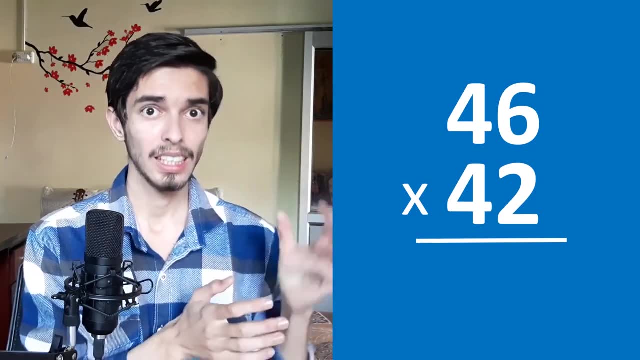 in this problem. So 46 multiplied by 42. Now think most of you can't even do this mentally. but here we are going to do it in 3 different ways. Now, before doing this, I just want to tell you the. 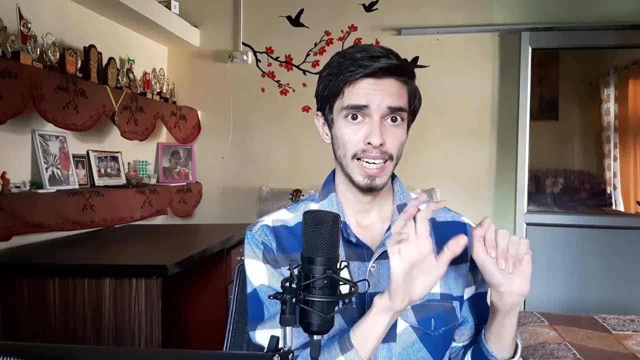 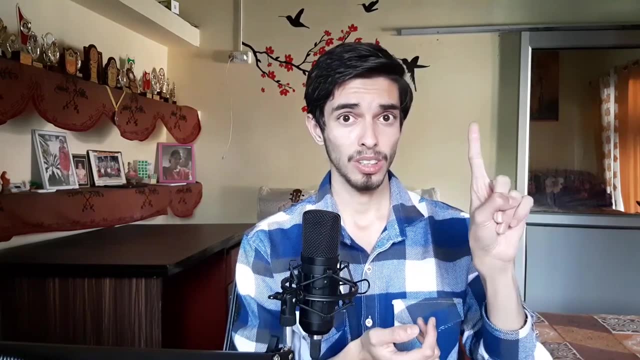 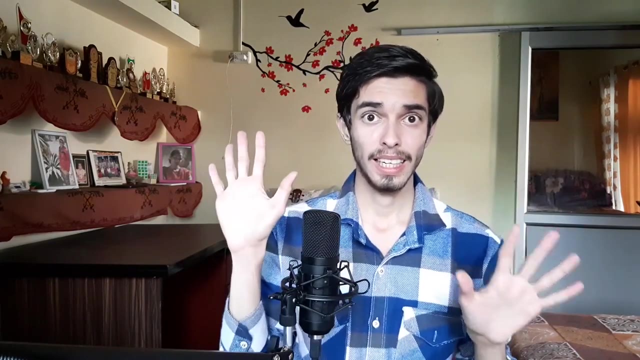 rule of thumb with which you can store numbers in your hands, which would be really helpful in doing these 2x2, 3x3 extra problems. this is extremely simple. so this is 1,, this is 2,, this is 3,, this is 4,, this is 5,, 6,, 7,, 8 and 9, you can store in this hand too. so 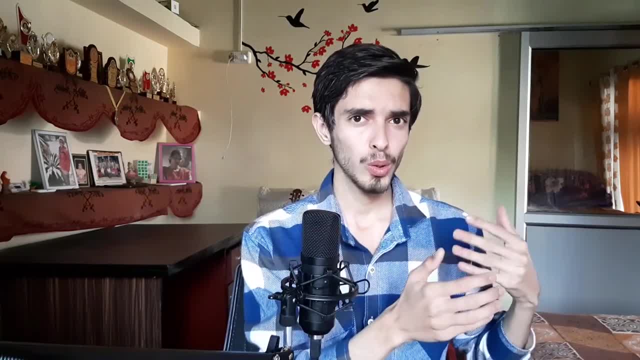 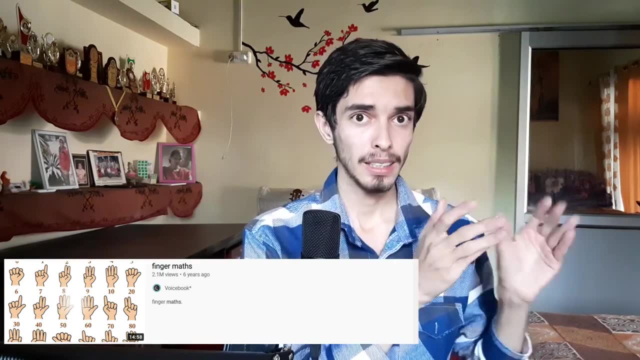 you can store 2 numbers in your hands. have you ever seen those videos in which students are doing like this, this, this, this and doing mental calculation? they are doing this same method, but a little advanced one. with their hands they are mimicking the abacus. 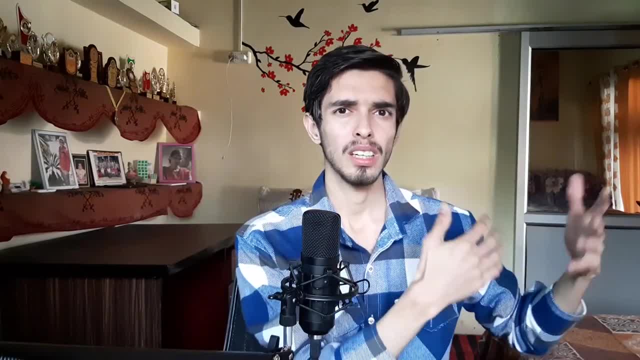 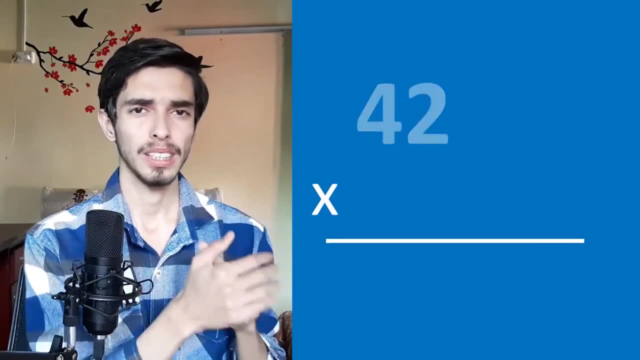 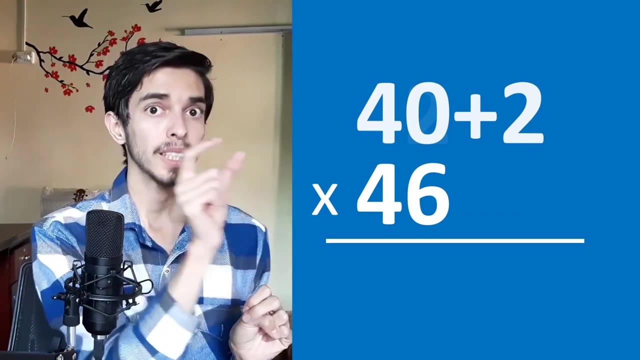 they are also storing numbers in their hand, but they are going to 100,000, so that is a little advanced method and a story of another video. so the addition method for 46 times 42, now 40, plus 2 times 46,. now store 2 in your hand like this: ok, so 40 times 46, which? 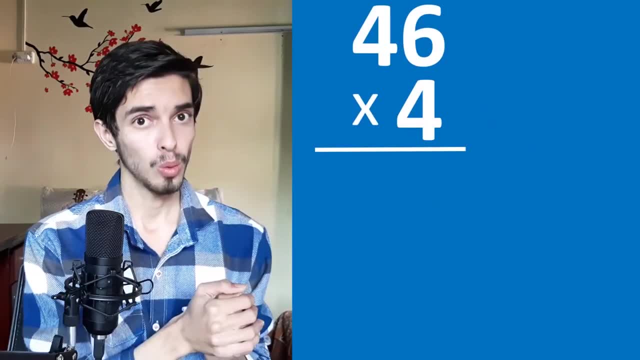 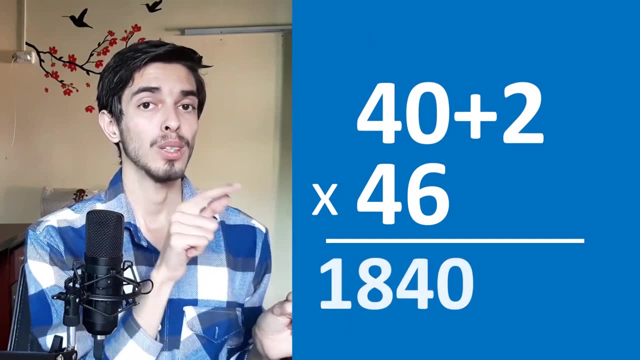 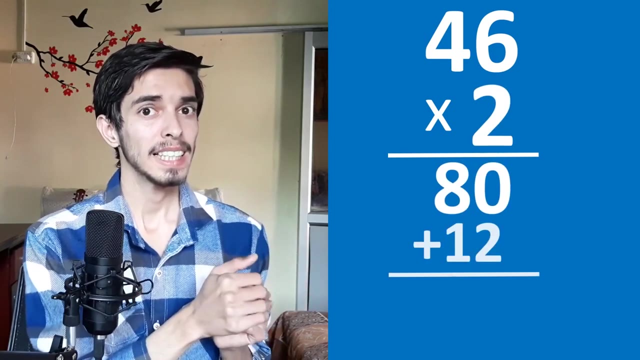 is just a 2x1 multiplication, so 46 times 4,. so 4 x 4 is 16,, 160 plus 24,, 184,, so 1840,. now 1840 plus 46 times 2, which is 92,, so 1840 plus 92, which. 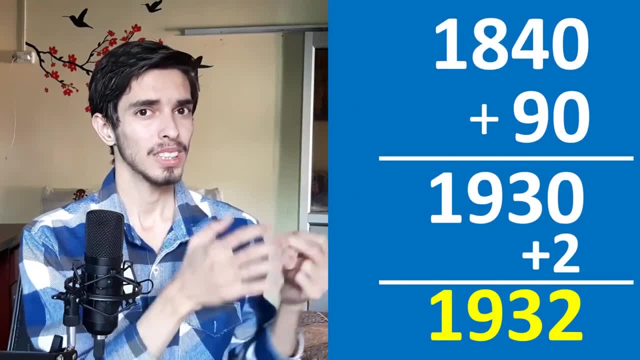 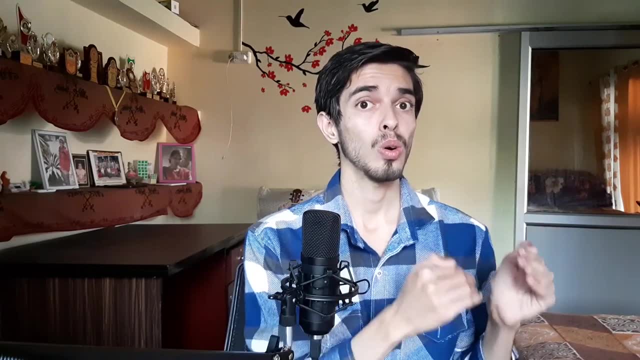 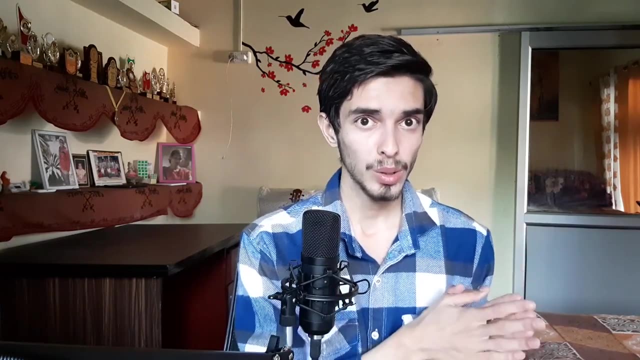 is 1932,. this is our answer. so this is how we can use addition method to solve problems, but this was not that easy. there were a lot of small problems that we had to do in this. so let's try the subtraction method for 46 times 42,, so 50 minus 4 times 42,, 4 in our 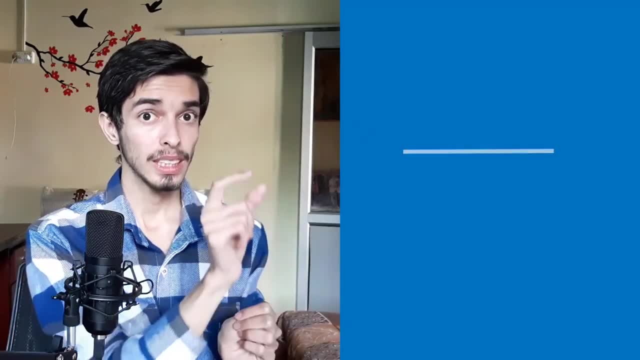 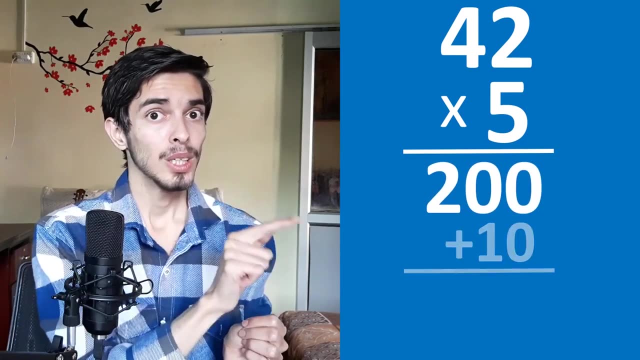 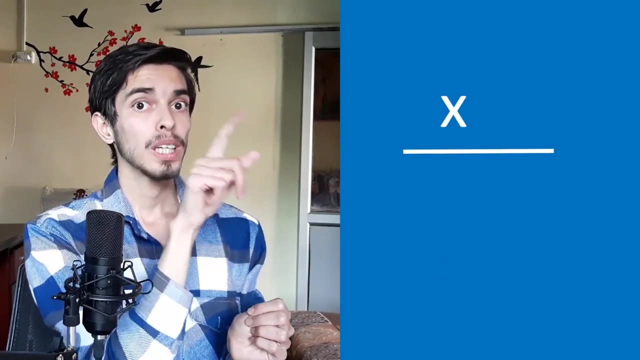 hand like this: so 50 times 42,, which is 5 times 42 with a 0,. so what is 5 times 42,? 5 x 4 is 20,, 5 x 2 is 10,, 210 with a 0,, so 2100,. now 2100 minus 4 times 42,. so what is? 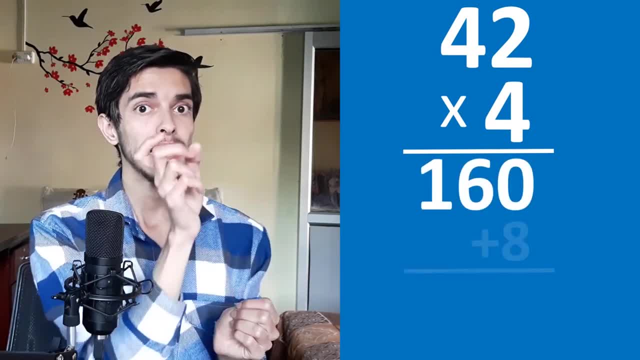 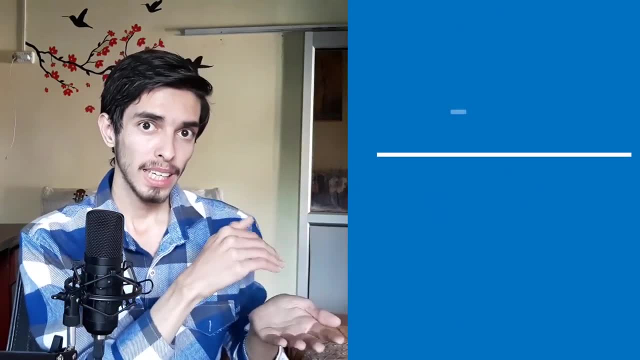 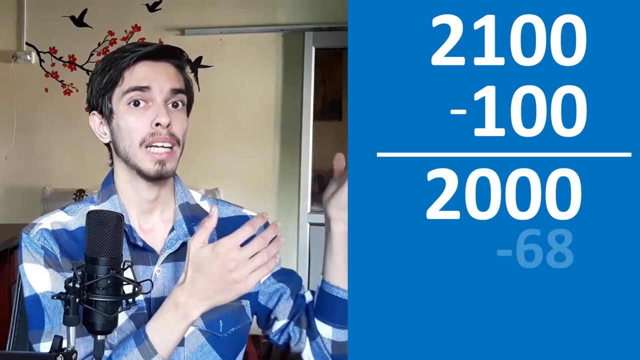 4 times 42? 16,. 4 to the 8, 168,. so 2100 minus 168,. now in here we subtract 100. first this is a basic subtraction problem. so 2100 minus 100 is what 2000 minus 68,. now in here we can be. 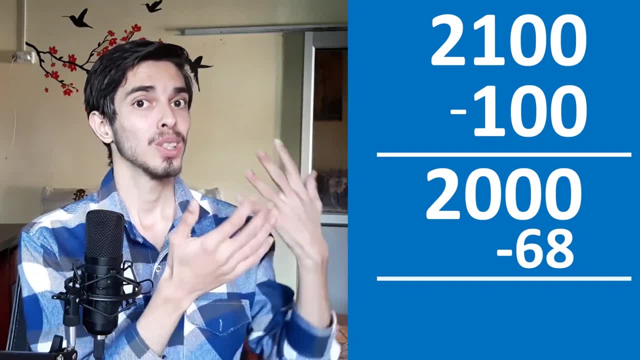 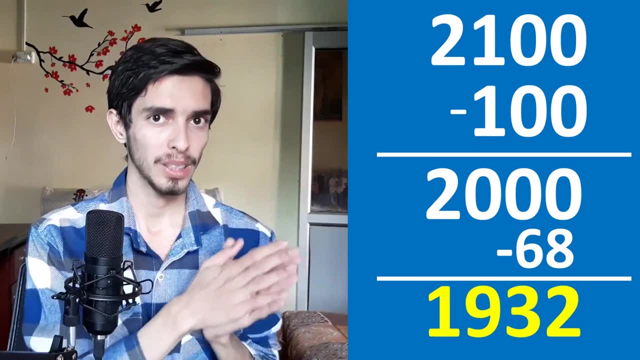 very cool with the complement of 68, which is 32, so the answer is 1932,. so this was the subtraction method for multiplication of 2 by 2.. This was easy, but not that easy. so let's see the factoring method for multiplication. 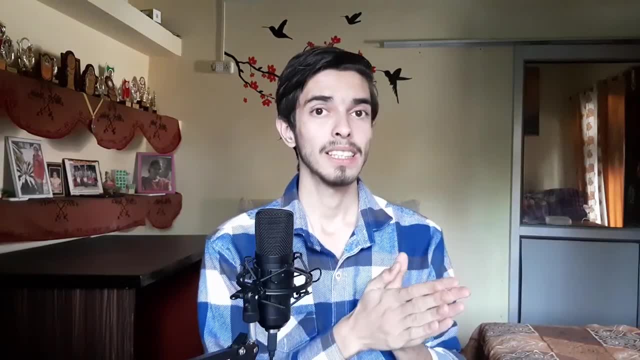 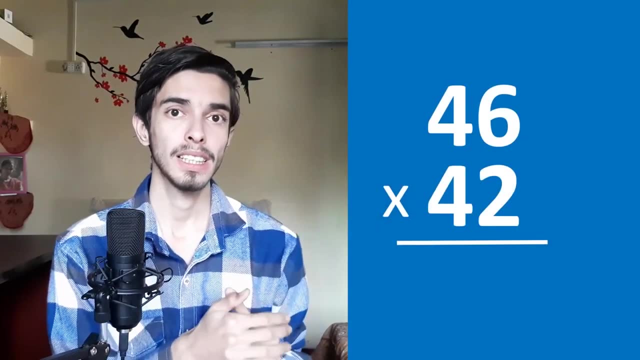 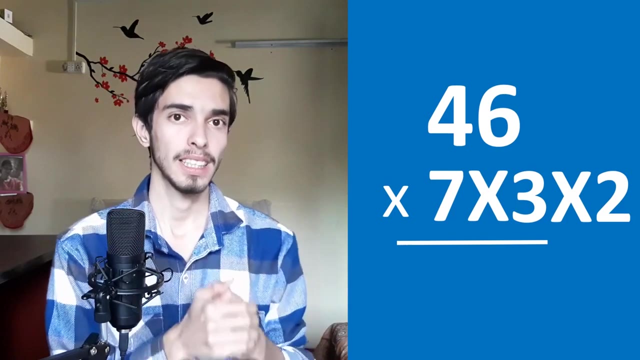 of 2 two-digit numbers. now, the factoring method is a really easy method, but it works only on numbers which can be factored like. we can write 42 as 6 times 7, and then also we can write 6 as 3 times 2, and this will make our multiplication really easy. so let's 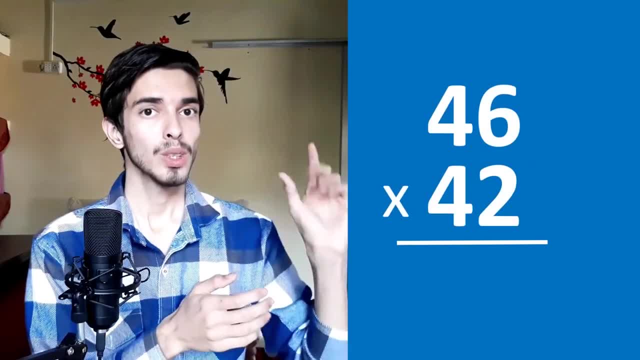 apply this factoring method on 46 times 42.. So 46 times 42 can be written as 46 times 42.. So let's apply this factoring method on 46 times 42, so 46 times 42 can be written as: 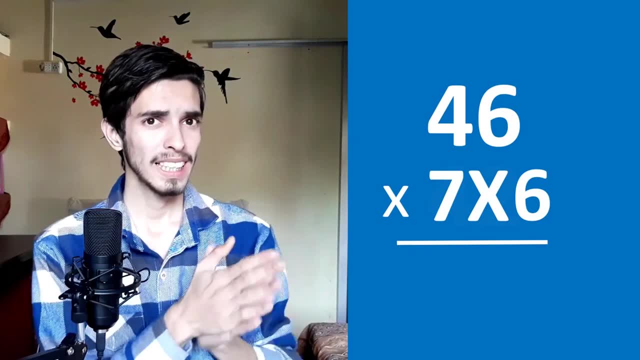 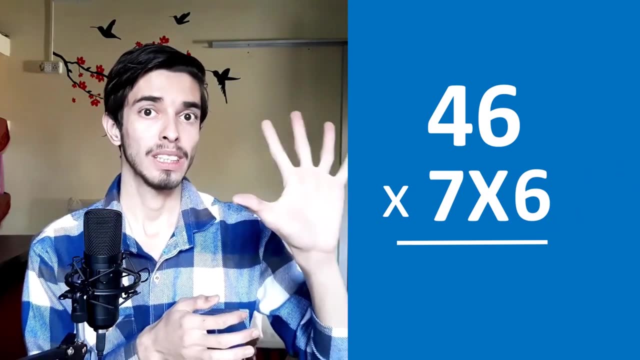 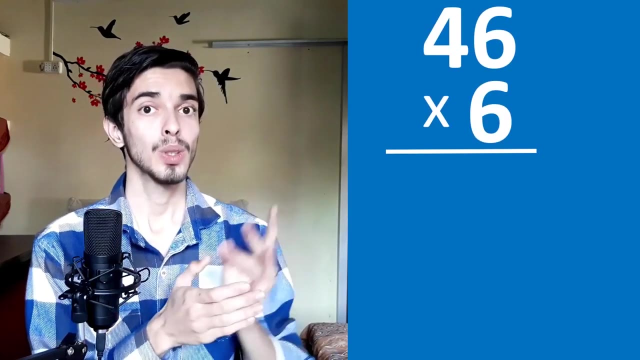 46 times 42.. We can also write 6 as 3 times 2, but let's not do that, because we know 2 to 1 multiplication very well. so let's store 7 in our hand. so 5,, 6,, 7,, so 7 here. so we have 46 times 6,. 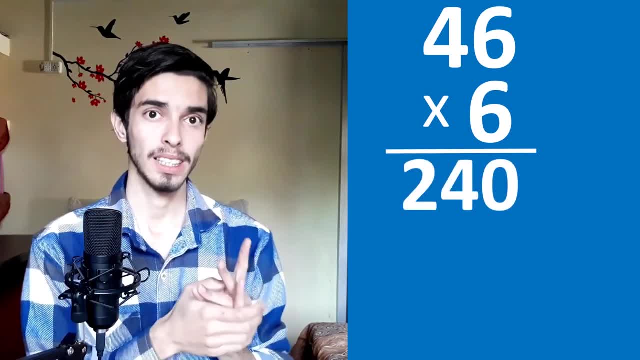 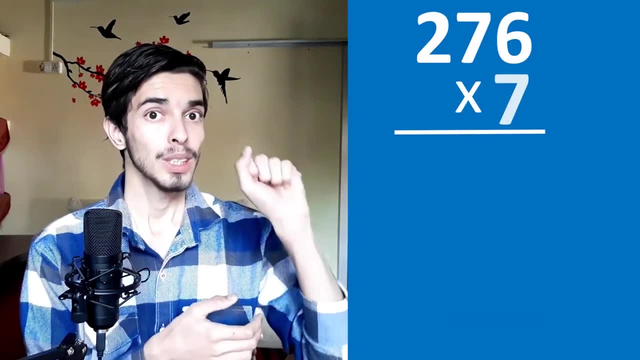 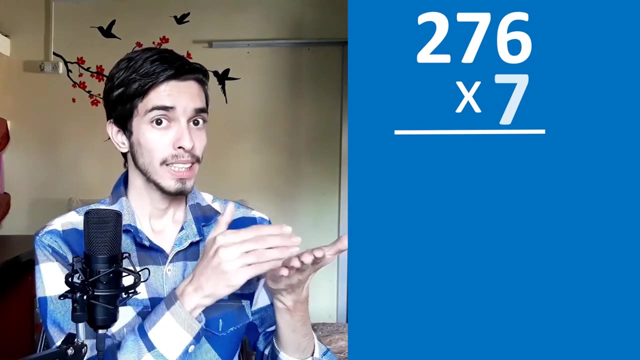 so 6. fours are 24,, 240 plus 6. sixes are 36,, so 240 plus 36,, which is 276, now we have 276 times 7.. So 276 times 7.. This is a 3 to 1 multiplication. so let's do it 276 times 7,. so 7 to the 14,, so 1400. 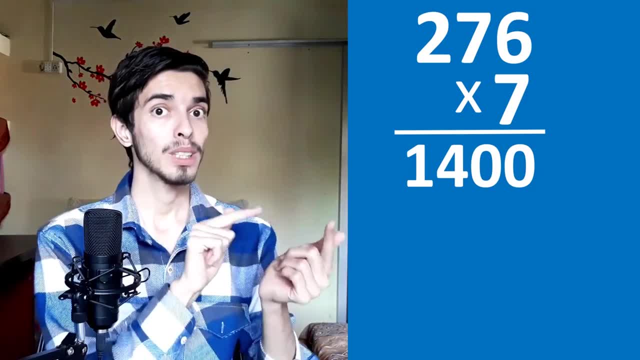 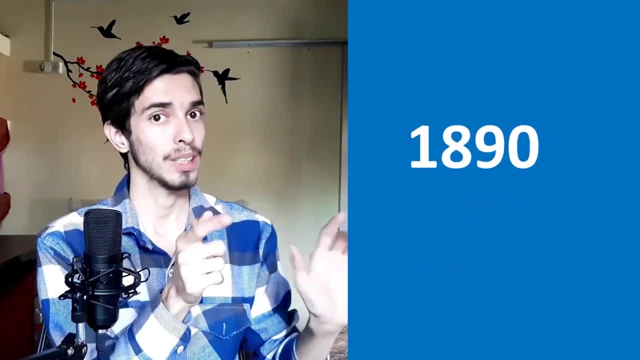 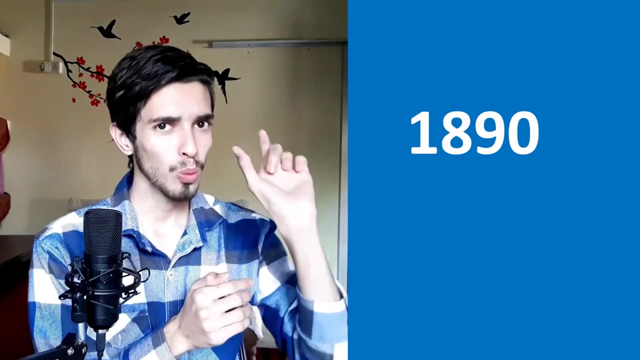 plus 7 times 49,, 1400 plus 49, and there is a 0 also, so 1400 plus 490, which is 1890,, okay, 1890,. now you have to say it again and again: 1890, 1890,, so 1890 plus there is a. 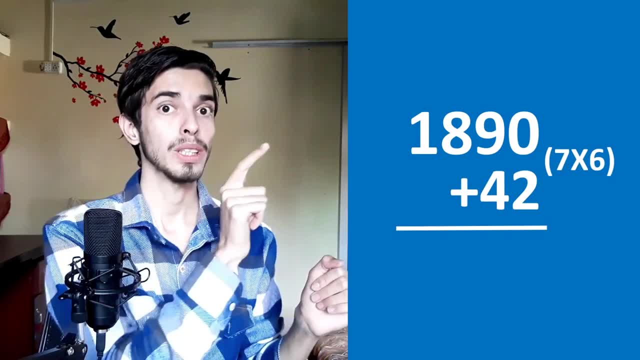 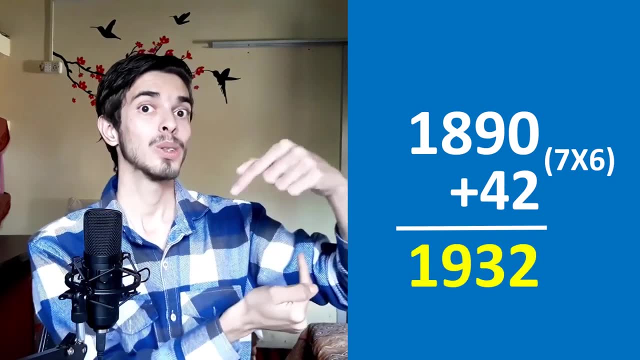 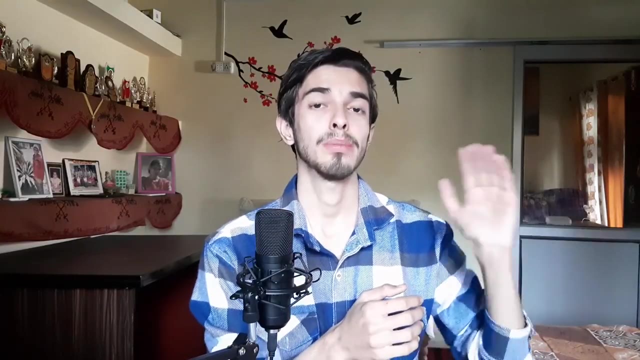 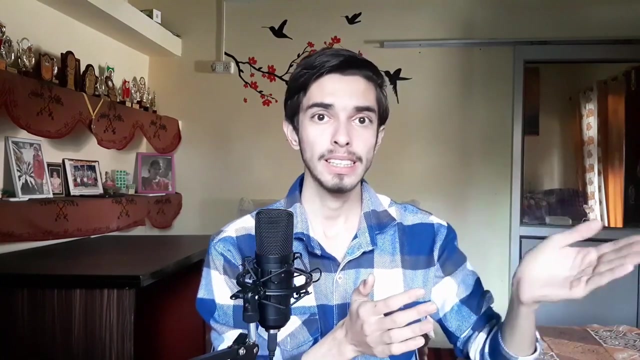 490.. So this is our answer. 1932 is our answer now. this factoring method was way easier than addition method and subtraction method, but this also depends on the problem that we have. sometimes subtraction method works best, sometimes addition and sometimes factoring method. so 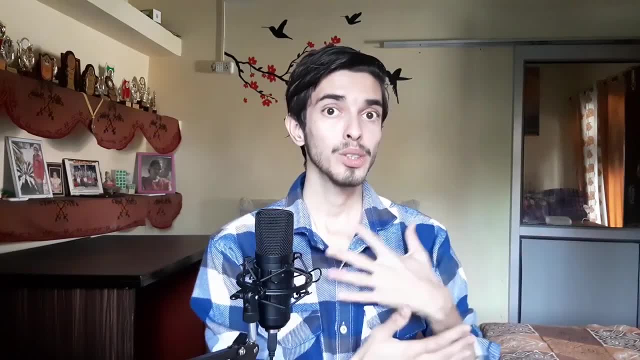 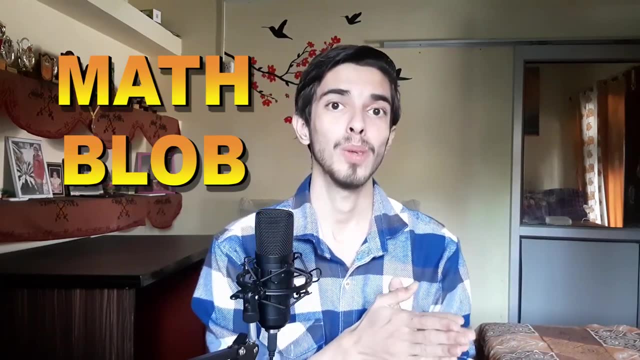 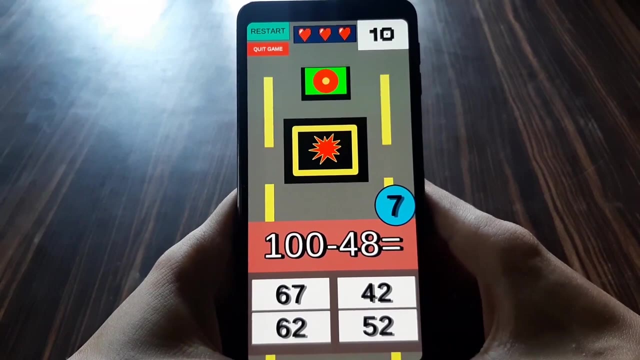 it depends on you that which one you want to use, And you will understand it automatically the more you practice. and for practicing I have specially made a game named Math Blob Run. in this game there is a good blob and there is a bad blob. chasing that blob who wants to eat it and solving math questions. 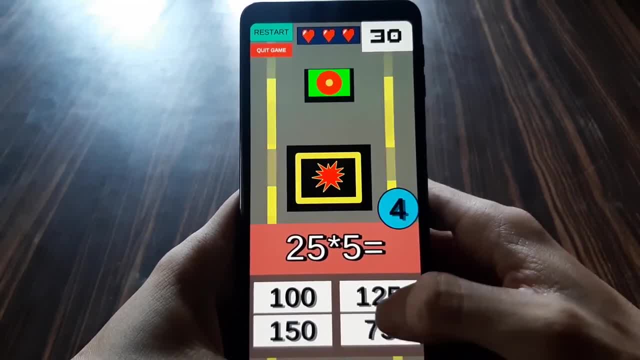 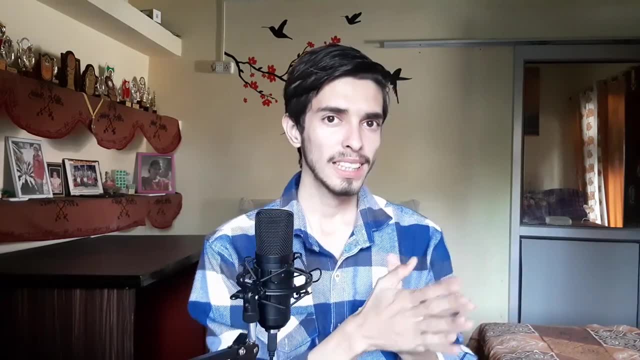 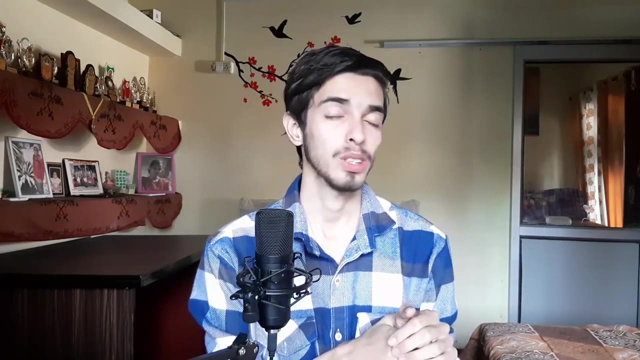 the mental math questions will save your blob, so this game will help you to practice mental math. download link of this game is in the description of this video. Now let's learn that legendary criss-cross method. For this you need a pen and paper, but don't worry, your mind won't rest. 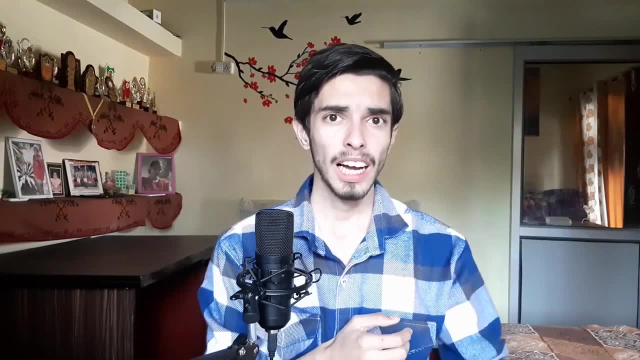 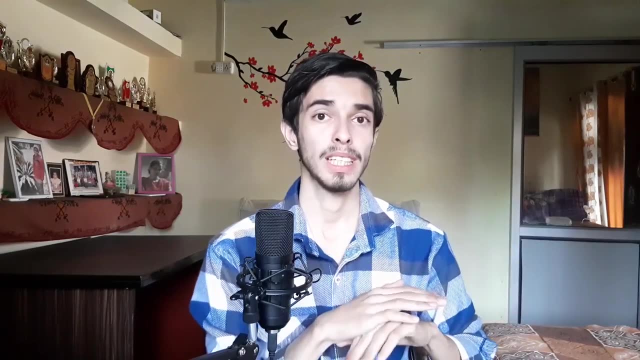 When in this book I was going to learn this method, I thought that after learning this I will be like Shakuntala Devi: I will be able to solve long multiplication problems really fast. but just wanna tell you this method is nothing special, it is just a different. 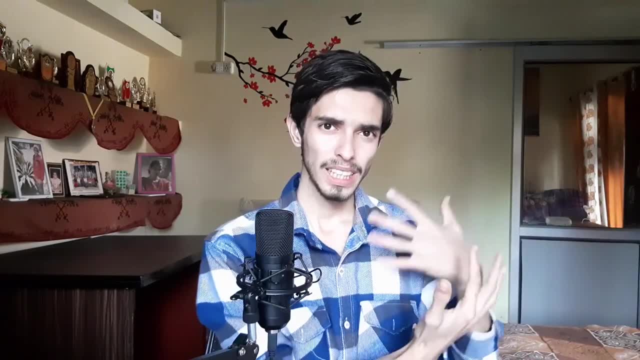 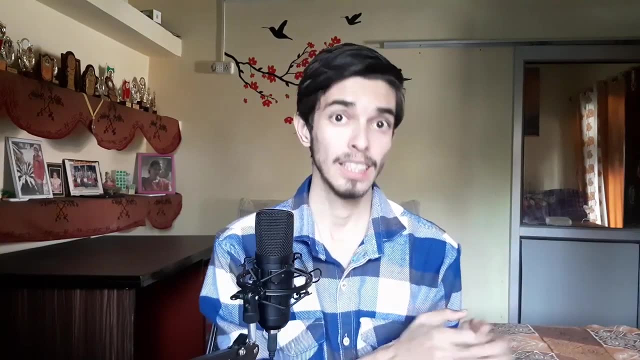 way to see multiplication problems, But it is way easier than the method they teach us in school. but on the other hand it also won't make you a super smart. With practice you can get better at it, like Shakuntala Devi. 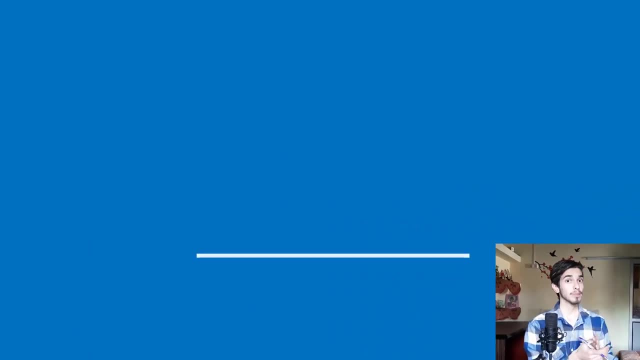 So let's learn the criss-cross method. So 47 times 34 using the criss-cross method. So write 47 times 34 on paper like this. Now draw a line like this: So 7, 4s are 28,. write 8 in here. you can also write the 2 on paper or you can store it in. 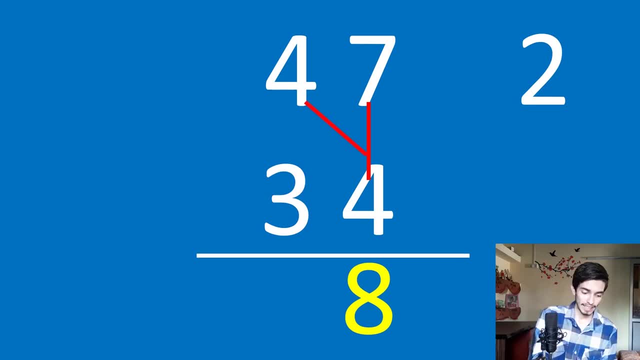 your hand like this. Now draw a diagonal like this: So 4- 4s are 16, and in this 16 add this 2, so 16 plus 2 is 18, now 7- 3s are 21.. 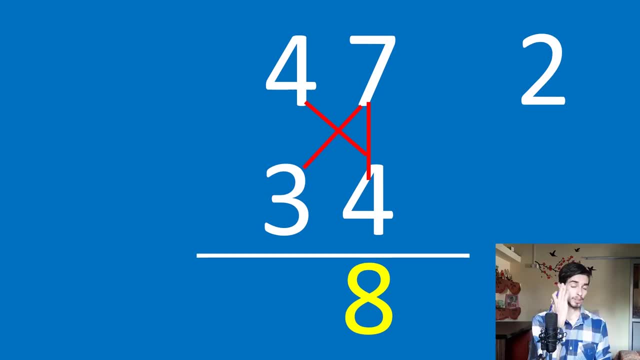 So 21 plus 18,. now you can do this mentally or write it on paper. I will prefer to do this mentally. So 21 plus 18 is 21 plus 10, which is 31,. 31 plus 8 is 39,. so write 9 in here and we have. 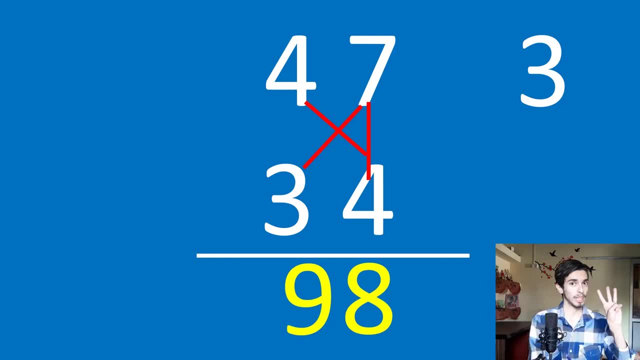 a 3,. now store 3 in your hand, or you can write it on paper like this: Now this one 4 times 3, so 4 times 3 is 12, in this 12 add 3, which is 15, so 1598 is our. 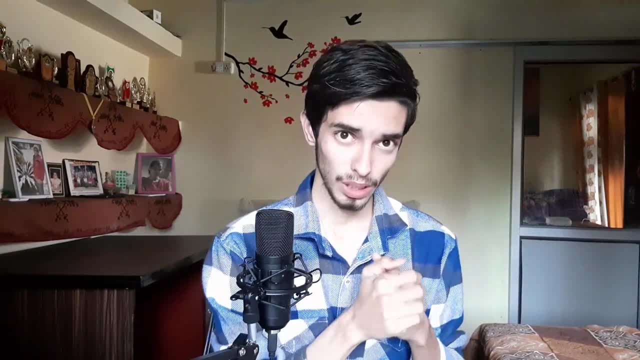 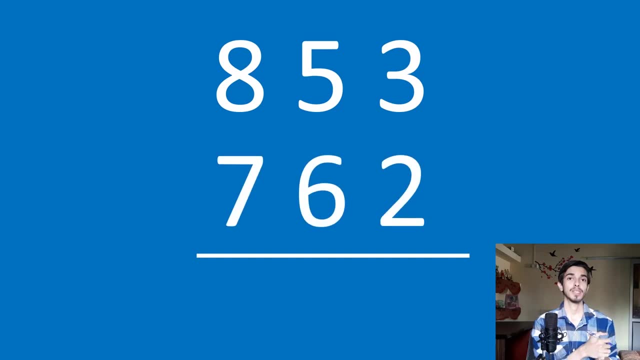 answer. So this is basically all the criss-cross method that you need to learn. Now let's try it on a 3 x 3 problem. So 8, 53 times 762, using the legendary criss-cross method of pen and paper. so write them like: 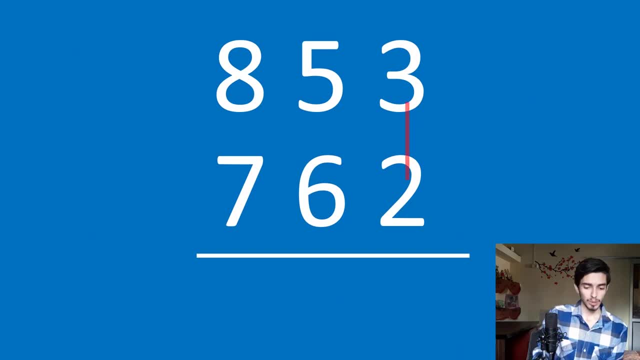 this 8, 53 times 762.. Now 3, 2s are 6,, now carry 5. 2s are 10 plus 6, 3s are 18,, 10 plus 18, 28,, 8 in here and 2. 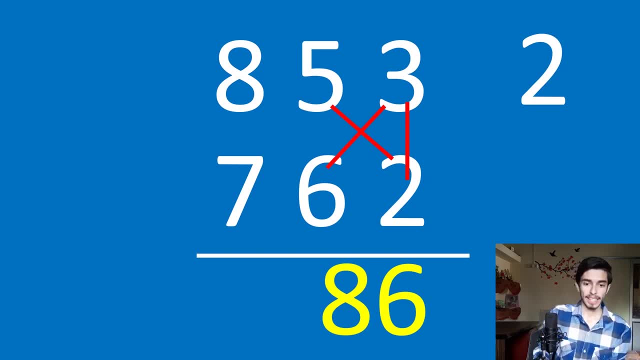 in your hand like this. Now you need to take a longer diagonal. So 8: 2s are 16,, 16 plus 2, 18,, 18 plus now center 6: 5s are 30,, 30 plus that 18, which 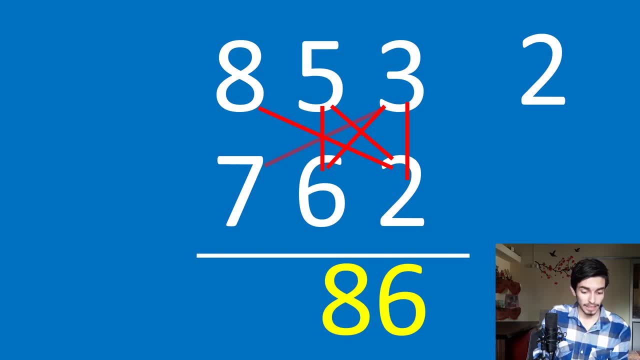 is 48.. Now remember 48, 48 plus 7, 3s are 21.. 48 plus 21 is what. 48 plus 20 is 68,. 68 plus 1 is 69.. So 9 in here, like this, and 6 in your hand, like this, or on paper, whatever you choose. 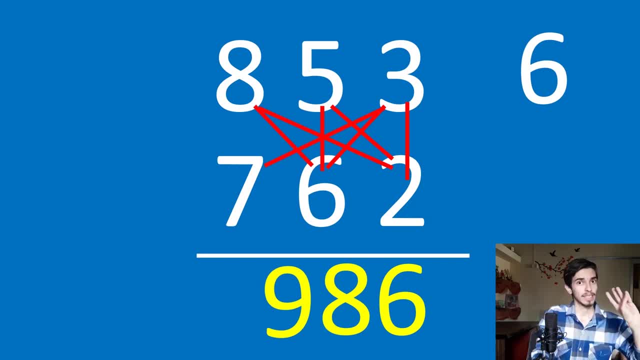 Now 8: 6s are 48,. 48 plus 6 is 54,. 54 plus 7: 5s are 35.. Now 54 plus 35, this is a longer addition problem. 54 plus 30 is 84,, 84 plus 5, 89.. 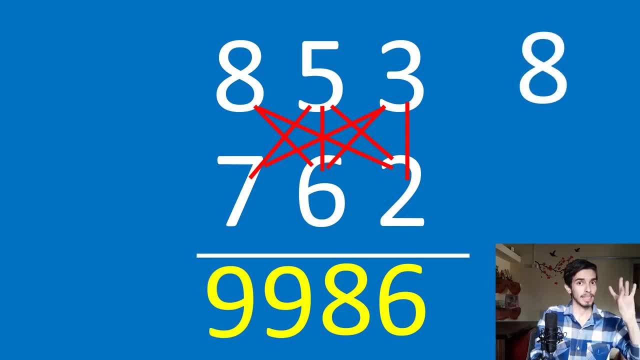 So 9 in here, or you can store 8 like this: 5, 6, 7, 8, now 8 in here. So 7: 8s are 56, 56 plus 8 is what 64.. So this is our answer: 649986..